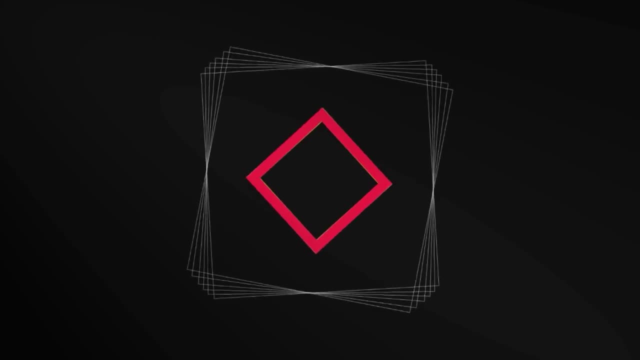 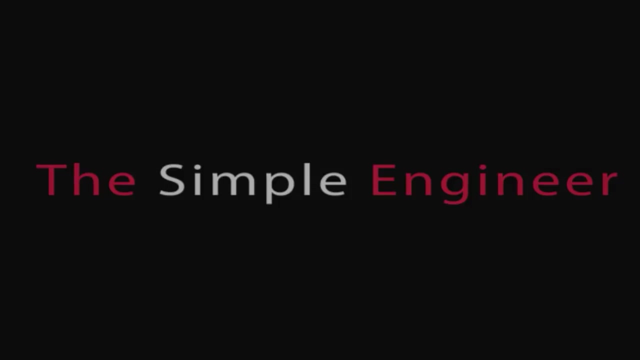 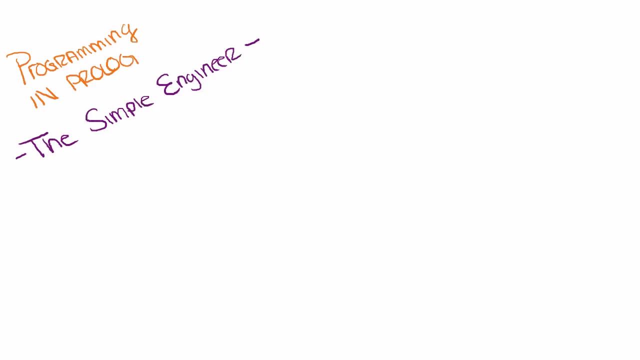 What is going on, guys? Welcome to a video slash micro lecture brought to you by The Simple Engineer. Today we are going to be delving into the topic of the prologue programming language. So, to begin, we're first going to want to download two pieces of software. They're both. 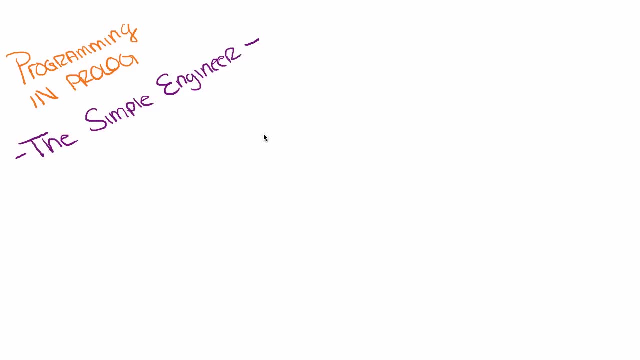 free, both cross-platform. The first one is going to be the text editor, and it is called Sublime Text, and the second is the IDE, which is called SWI Prologue, and this will be used to compile and run your prologue code. Okay, so many of you may be asking what is prologue? Well, 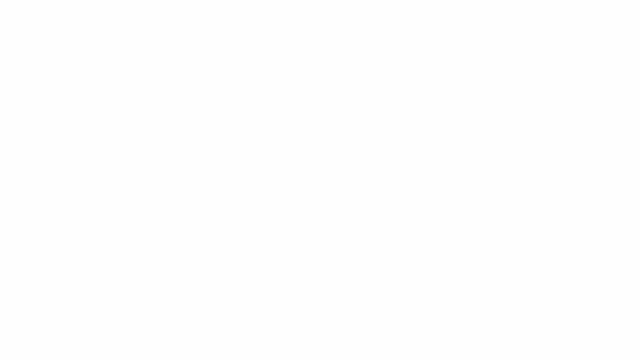 prologue falls under the paradigm of logic and it's a declarative programming language, and what that means is that it kind of gets rid of programming. and prologue itself uses something known as predicate logic or predicate syntax, and it's similar to that of the natural language. 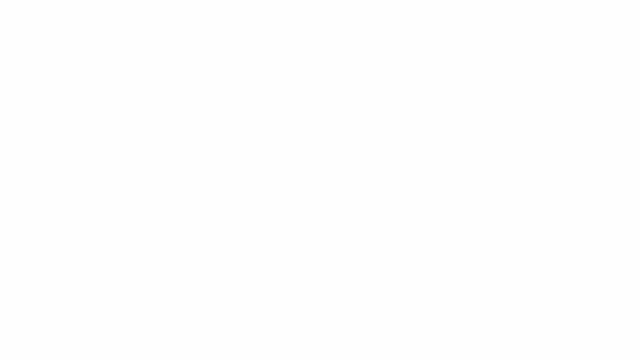 and it was developed to more easily convey ideas. So three things that I want to cover in this video, since we're kind of short on time, is: first, we want to cover what facts what facts are. We want to cover what rules are, and then we're going to delve into the compiler, write some code. 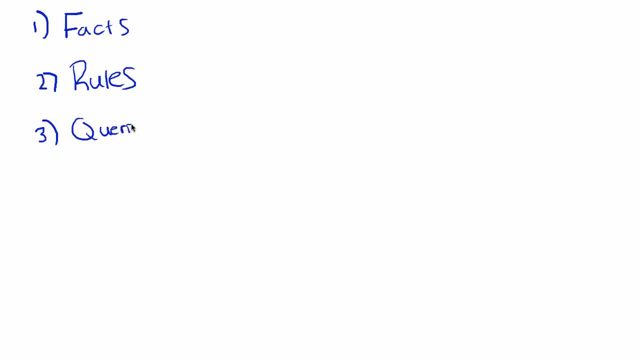 and cover what queries are Okay. so first things first. let's go ahead and look at facts. So facts are basically just what is known. They're just axioms about some objects and their relationship. So we'll go ahead and give a couple examples of that. So say we have a couple facts, Let's 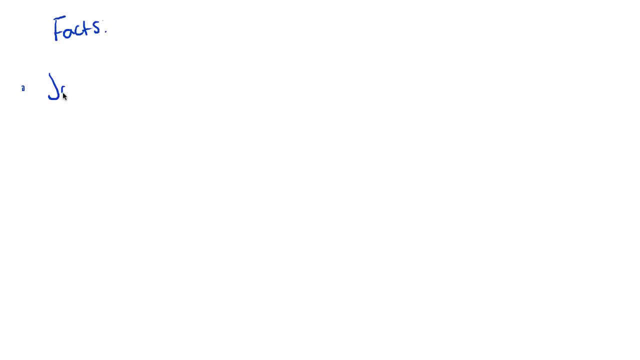 say: our first fact is Johnny is fat. We have another fact called the dog is brown, Susie likes Bobby, etc. etc. idea, these are facts. now we want to convert this to predicate logic in terms of prologue to understand. so we take the predicate, so let's highlight the predicates. we have fat we have. 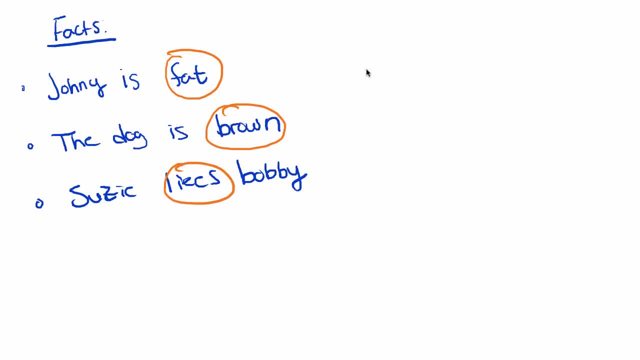 brown and we have the likes. so to convert this in terms of prologue, we would say: what is fat? well, johnny's fat. and then we end this fact with a period. this is how every expression or fact is ended in prologue. then we would say: what is brown? well, the dog is brown. 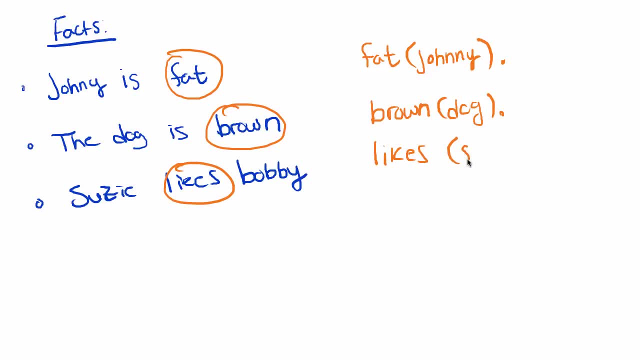 who does who like likes susie, susie likes bobby. so here the only difference is there's two arguments and the predicate, so the predicate satisfies two arguments. now something to note is the name: the Hao and the Hu, so the name. i come into the picture for all, all orders of trade with this. 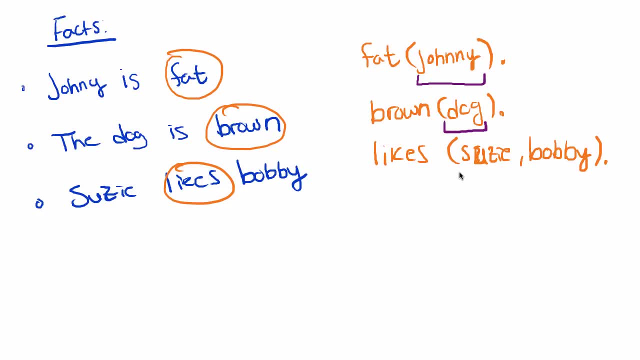 is the name of the dog buzz and it says multi-title. so okay, if we start gros to mean whether, if you number of arguments here, so you see one argument, one argument, two arguments. this is known as the arity, so if you see the number of arguments or something referred. 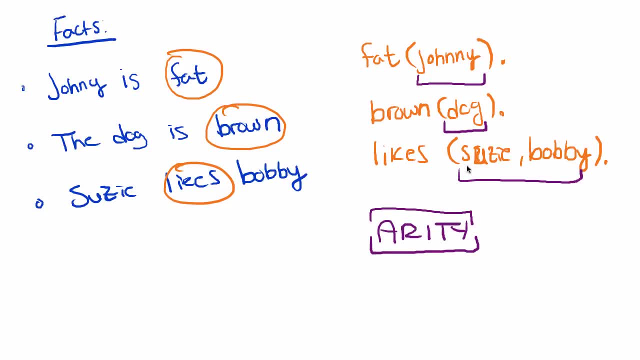 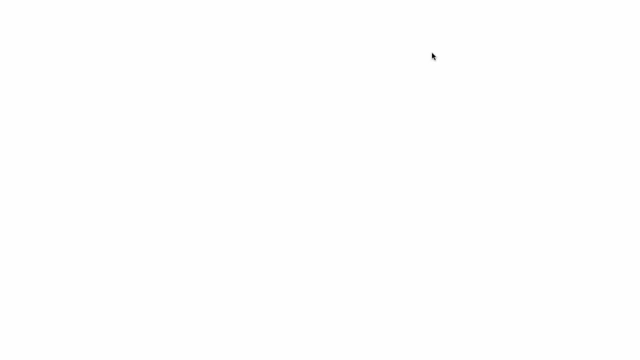 to as arity, that's, the number of parameters or the number of arguments passed in this type of constructor. okay, next thing we want to look at are rules. now, rules just extend the facts about objects and their relationship. they really enable you to infer facts from other facts and a more simpler 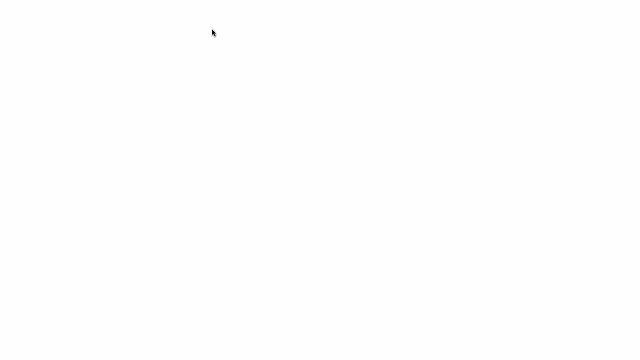 explanation. so let's go ahead and look at an example for rules. okay, so we say that let's give an example we know. let's say that we know that we have a rule that says that we have a rule that says that we have a rule that says that's good for the other random variables, Say: 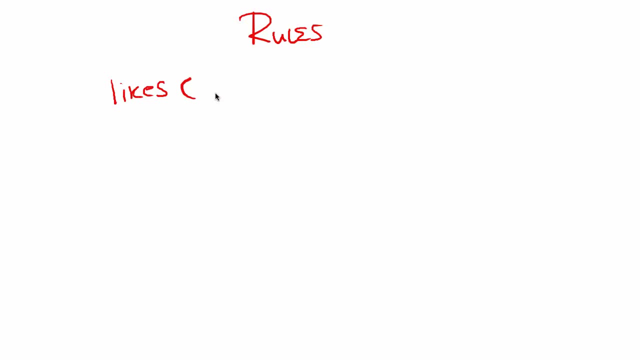 manouche andева of neыт, cut out and veyent an wrestual interval. what would that say to me? let's say Ryan likes- we should actually be lowercase. we'll talk about that a little bit. let's say Ryan likes Britney. 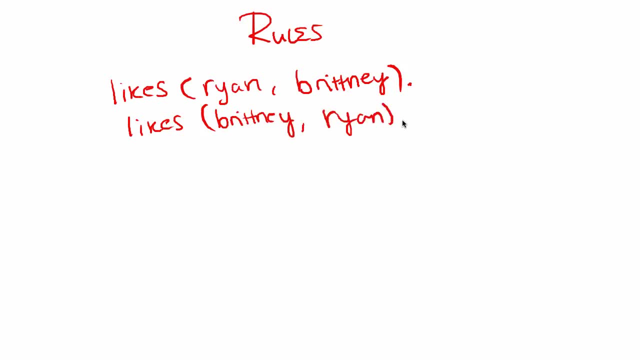 and it and we'll say Britney likes Ryan. and we'll do a final one, say Dan like Josh. okay now, now we see that these people like each other's friends, but we want to know if they're dating. so we're gonna create a rule to better understand. 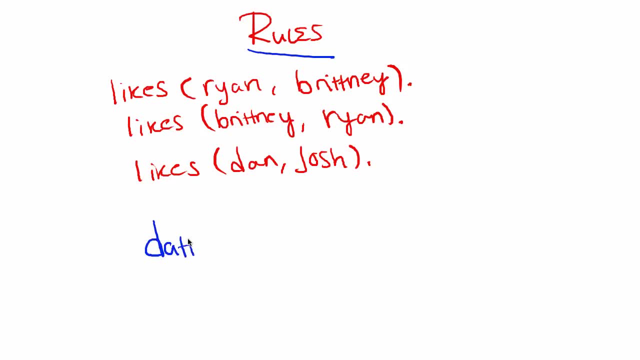 this idea. so we'll create a rule called dating, and it'll involve person X and person Y, and person X is dating person Y, and likewise if and only if, which is denoted by the logical implication of a colon and a hyphen: if and only if person. 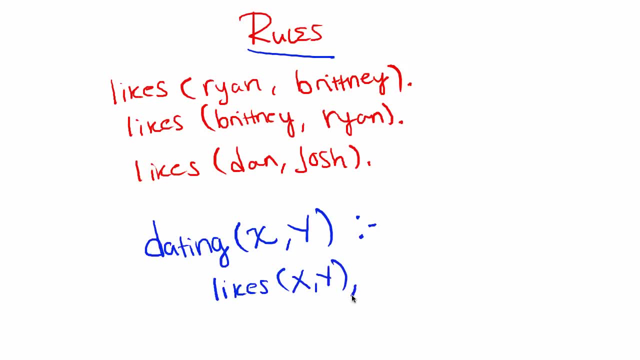 X likes person Y and person Y likes person X. okay, so there's a few things to note here that may look a little strange. first of all, what is this logical implication here? well, there's actually a column of rules that you should know about the rules that you should know about the rules. 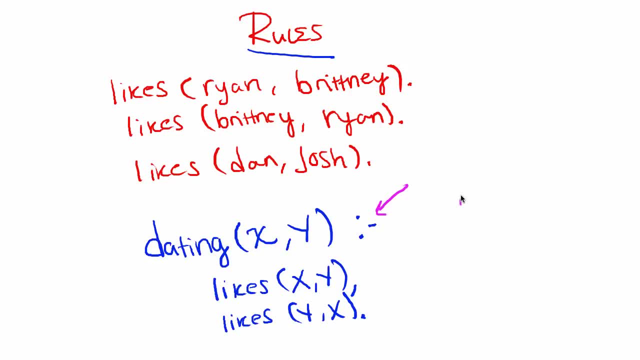 that you should be aware of. first of all, you know, in programming we have and statements, we have if statements. we have or statements and we have not, or negated statements. so the equivalents for all of these will be denoted by the following: and statements are always denoted by a comma, if statements are denoted by a. 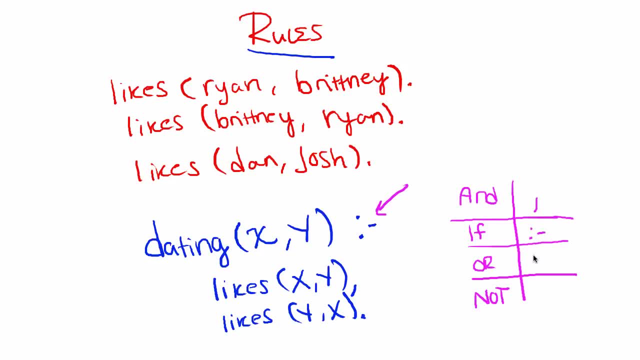 colon and a hyphen, or statements are denoted by a semicolon and not statements are denoted by the English term, not okay? so here we're saying person X, which is capital. so remember that all variables are capital letters or capital words. so we're saying person X is dating. 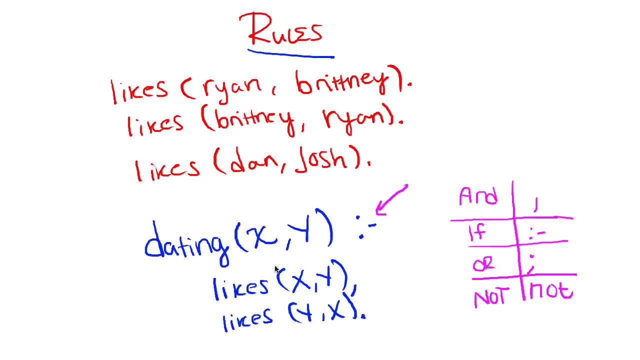 person Y, if, and only if, person X likes person Y and person Y likes person X. if all of this is true, then the output of the compiler should return true, else it would return false. okay, so now we've covered rules, so let's go ahead and jump into queries. 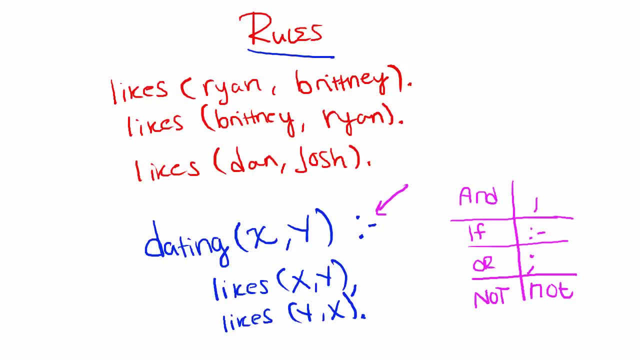 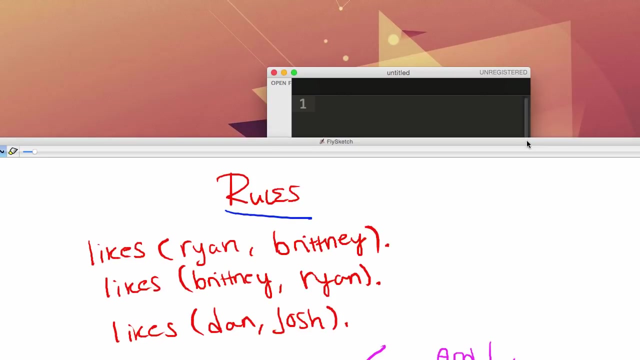 queries will combine the ideas of facts and rules together, except we will now be using the compiler to exemplify this idea. so let's say: let's see, here I'm gonna go ahead and open up sublime, and where is text? okay, so go ahead and open up sublime, or? 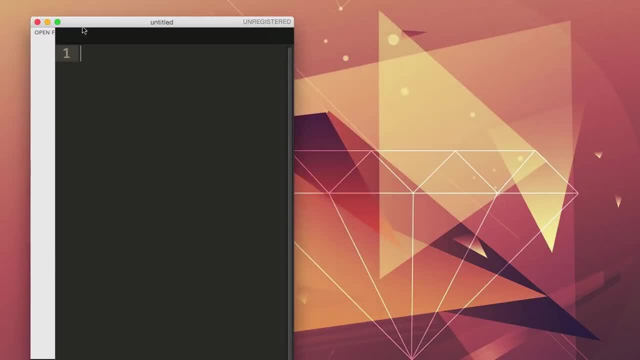 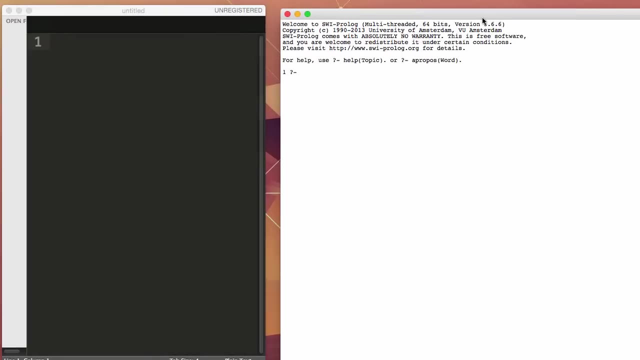 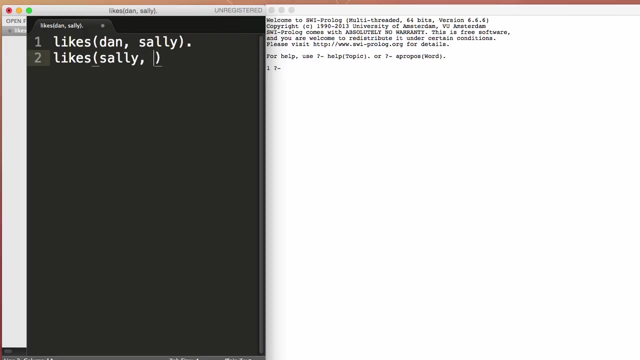 your preferred text editor and also go ahead and open up SWI prologue, which is the compiler. okay, we made a couple couple rules here. we said: Dan likes Sally, Sally likes Dan and Josh likes Brittany. okay, then we'll create a rule and we'll say: dating person X, dating person Y if, and only if, 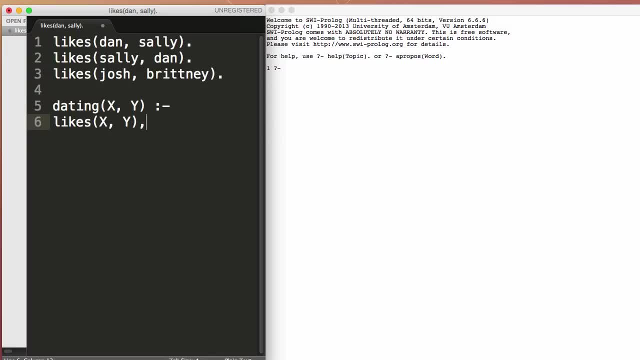 person X likes person Y and person Y likes person X, and then we'll create a- uh, let's say we'll create a rule called friendship of X and Y. so person X is friends with person Y if, and only if, person X likes person Y or person Y likes person X. 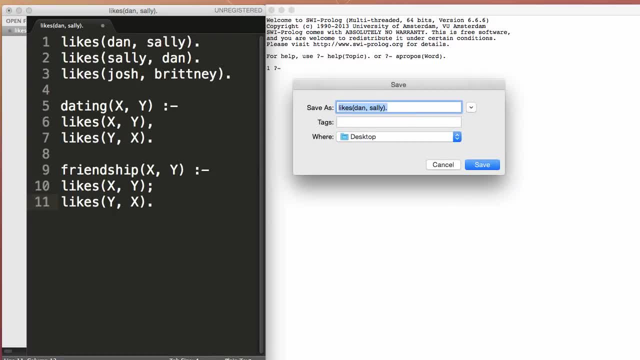 okay, so we'll save this to your desktop. the extension is dot PL for prologue, so we'll say testingpl and I'll go ahead and replace that. now, to run this, you just go opening left bracket, single quote type, in the location of the file mine's on my desktop, in single quote, in right bracket, period, and this ends the statement. 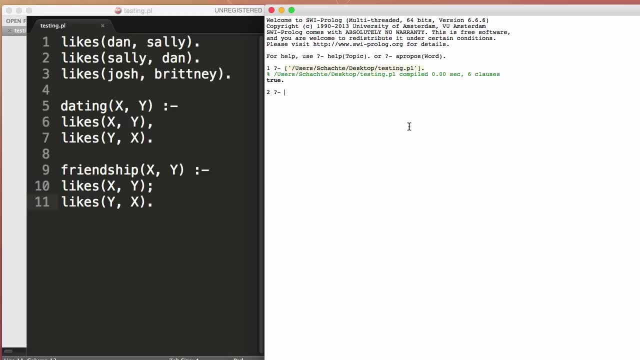 I'll go ahead and hit enter. there are no compilation errors, which is good. so now we can actually start querying. so to query, we'll say: let's see. okay, you see that there's a question mark here in the compiler. so it's saying: basically ask a question. and my question is: does Dan like Sally? 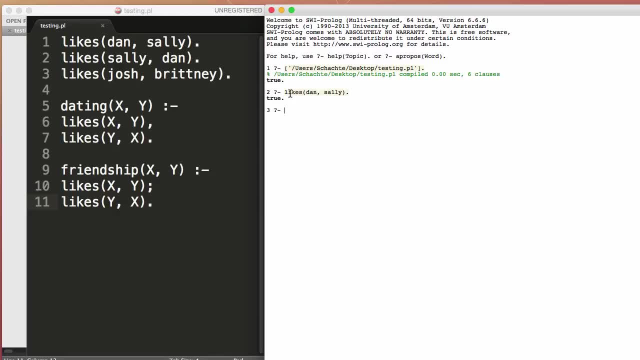 okay. well, this is true because in our fact base or in our database, Dan does like Sally. okay, so we can say: likes Blake, comma Josh: okay, well, this is false because we haven't defined in our fact base or database that Blake likes Josh. okay, now we'll jump into the rule and we'll say: okay, we want to know. 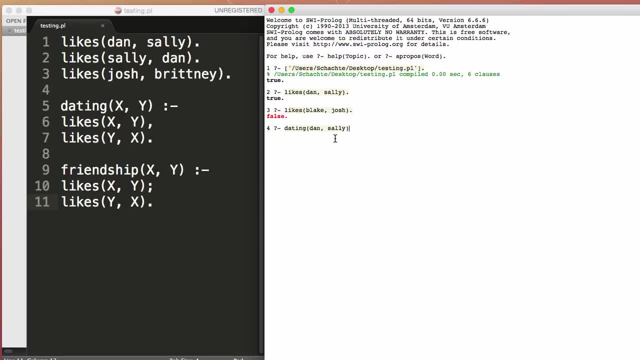 if Dan and Sally are dating, so we'll say Dan and Sally. this is true because Dan likes Sally and Sally likes Dan, and that satisfies what we have here now. Josh and Brittany are not dating, because Josh may like Brittany, but Brittany doesn't like him back. however, 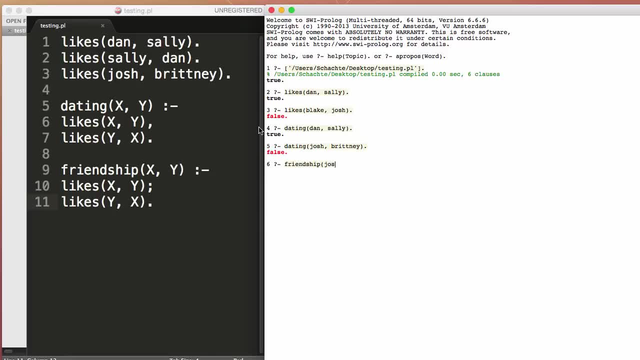 if we look at the friendship rule and we say Josh and Brittany, well, this is true, because here we say, okay, X has to like Y, or person Y has to like person X, and here we know that Josh does like Brittany, but Brittany doesn't necessarily like him back. 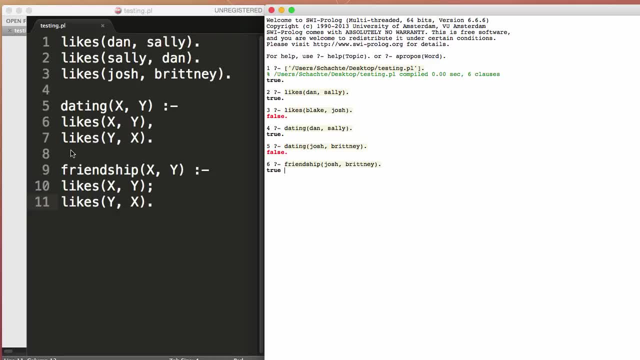 okay, so we've covered prologue facts, rules and queries and I've showed you guys how to compile and run your first prologue program. hopefully that gets you started. if you have any further questions, feel free to leave a comment in the bottom of the video and I will get back to you.